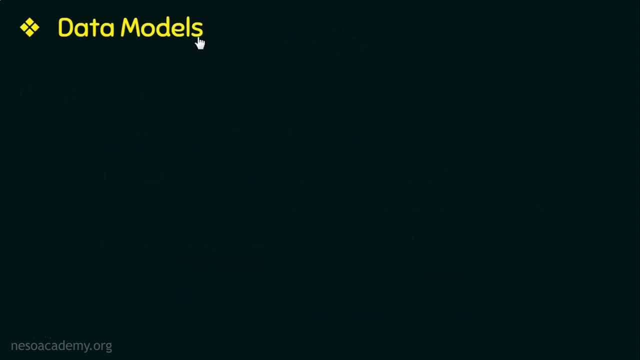 first, let us see what a data model is and why we require it. One of the most important characteristics of database approach is that it provides data abstraction. Now, what is data abstraction? Data abstraction is a data structure that is based on the data structure of a database. 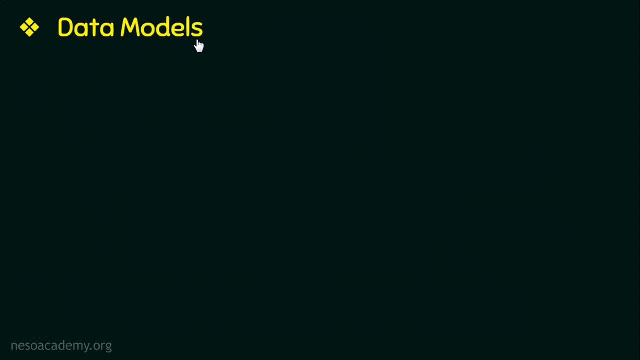 It is the hiding of complex details or details that are not needed by the database users. Now, to achieve this data abstraction, we have something called as data model. Data model is a collection of concepts used to describe the structure of the database, like specifying the data types. 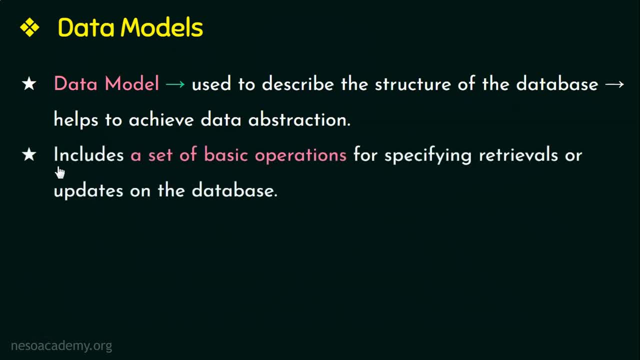 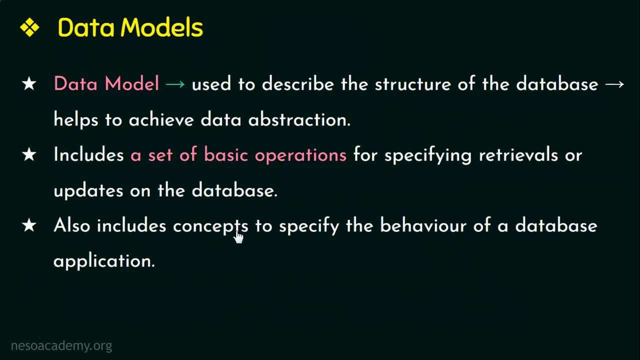 basic operations. data model also includes concepts to specify the behavior of a database application, And so it allows the database designer to specify a set of valid, user-defined operations. So this is an introduction to data models and why we require it. that is, to achieve data abstraction. Now we can. 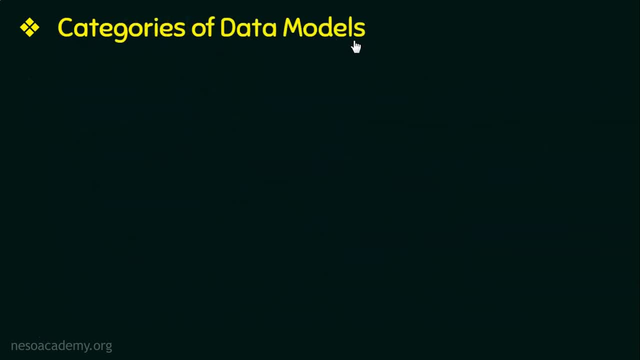 categorize these data models into a set of basic operations. For example, we can categorize the data vit, jakpl, rib on the database. no need to do it for now. these are the three main basic operations. The first category, high-level or conceptual data model, provides. 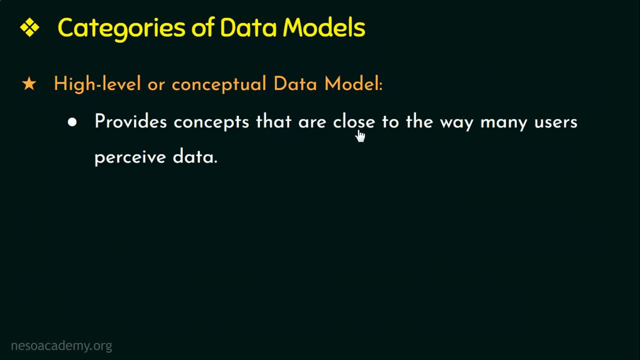 concepts to present data in a way or that are close to the way many users see or perceive data. The conceptual data models uses concepts such as entities, attributes and relationships. entities represent real world object or concept Like, for example, employee, student, etc. 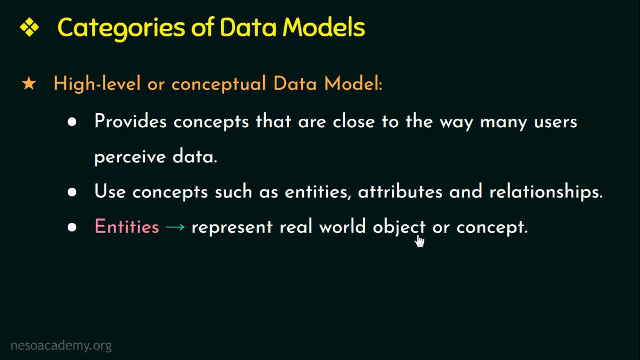 These are all entities as they represent real world. object. Next attributes: they further describe an entity, like the student name, role, number, etc. And then we have relationships, which is an association or a link among two or more entities, Like, for example, an employee works on many projects. 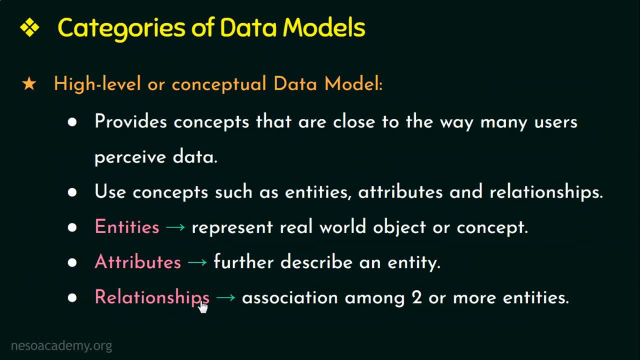 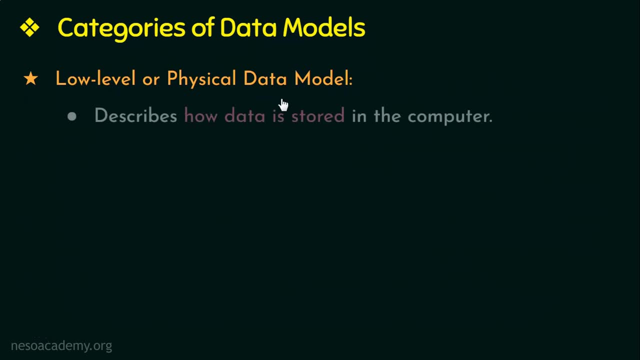 So a relationship exists between the employee and each project. So this is about the first category of data model, the high level or the conceptual data model. The next category is the low level, or the physical data model. This model provides concepts that describe how data is stored in the computer. 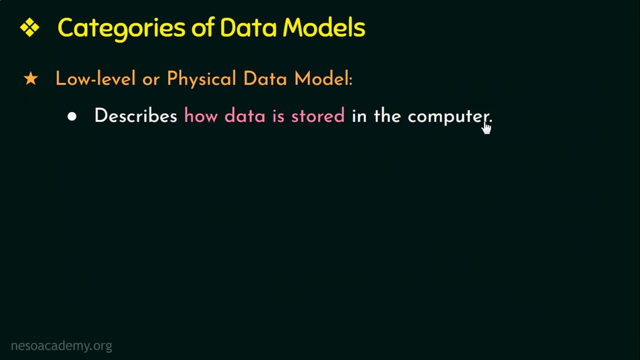 by representing information like the format, the access path, etc. An access path is a structure that makes search for a project, A particular database record efficient. or in other words, I can say: access path is a structure for efficient searching of a particular database record. 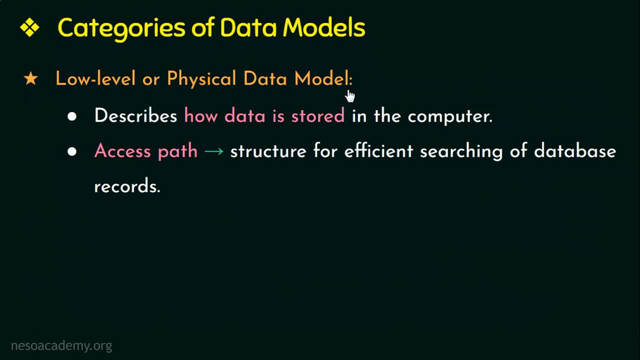 This is the second category, the low level or the physical data model. The next category of data model is representational or implementation data model. There are three data models that come under this category. The first is a relational data model, Then we have the network data model and the hierarchical model. 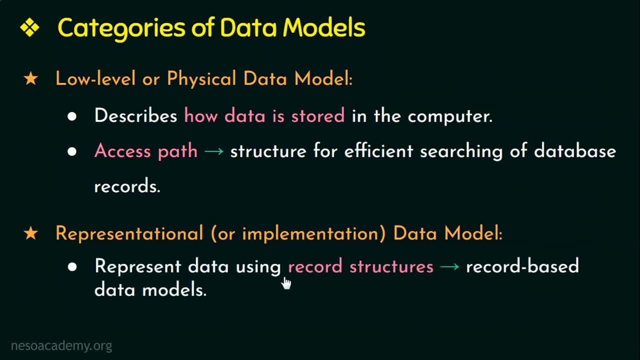 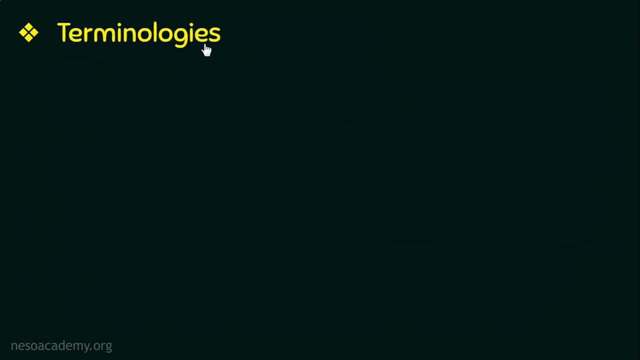 And representational data models represent data using record structures, And that is why representational data model are sometimes called record based data models. So these are the categories of data models. Next is the terminologies that we need to familiarize ourselves with. 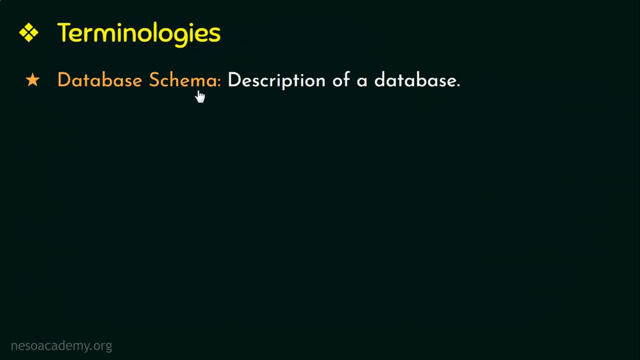 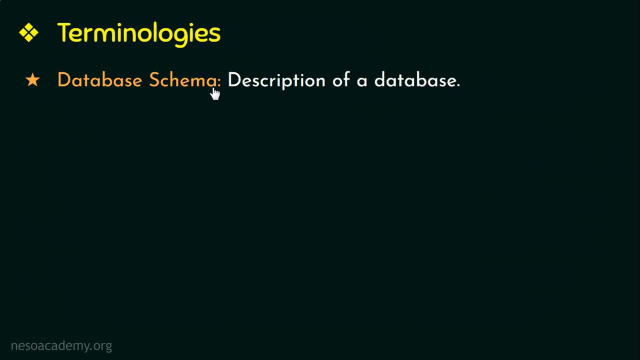 In our first video, we have seen that metadata is also a description of a database. Now, what is the difference between a metadata and a schema? Metadata is data about data, Or in other words, it describes the data in the database, Whereas schema is just a plan or a layout or a blueprint of the database. 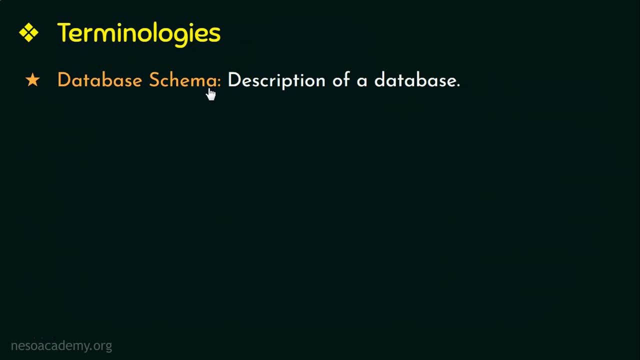 A schema is a subset of metadata, or it is one of the components of metadata, And a diagrammatic representation of schema is called a schema diagram, Or in other words, it is the displayed schema, And this is how a schema diagram would look like.